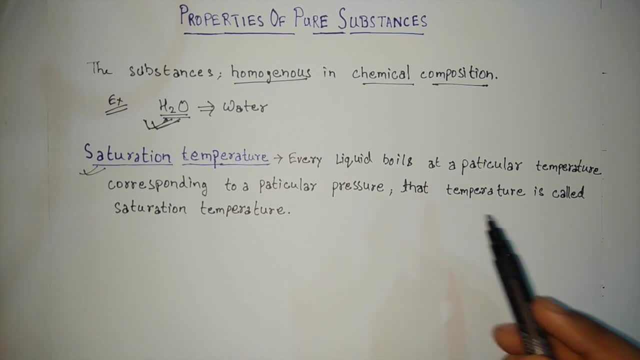 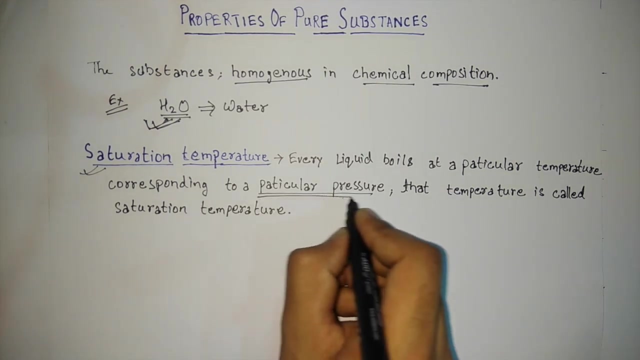 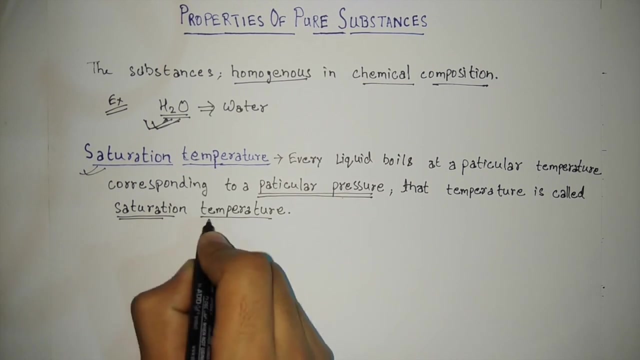 For every liquid. a liquid boils at a particular temperature for given corresponding particular pressure. That temperature is called saturation temperature And the pressure at which it is boiling it is known as saturation pressure. It is called the saturation pressure, and the temperature corresponding to this pressure is known as saturation pressure. As I told, 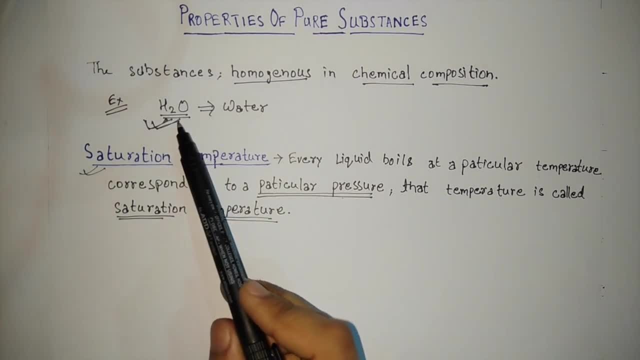 you. above that water- that means H2O- is an example of pure substance. so let's try to study the nature or the variation of pressure with respect to temperature of water. This graph shows the variation of pressure with temperature of water. This line is known as sublimation line, while this line is known as vaporization line, and 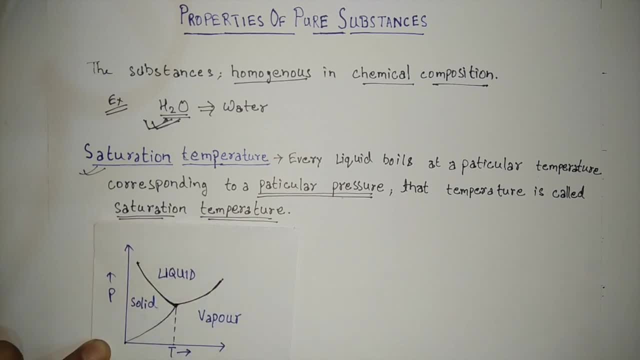 this line is known as fusion line. Between sublimation line and the fusion line, the solid state exist, and between the sublimation line and the vaporization line The vapor phase exist. and between the fusion line and the vaporization line the liquid phase of the water exist. 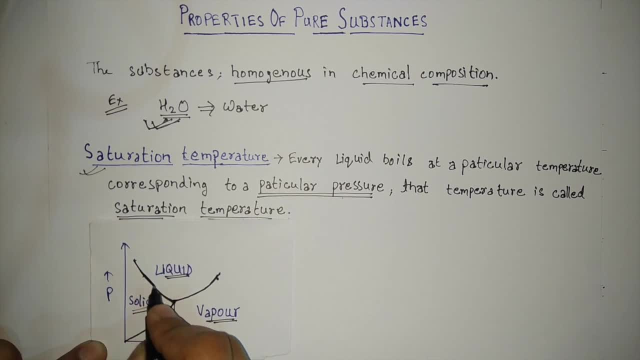 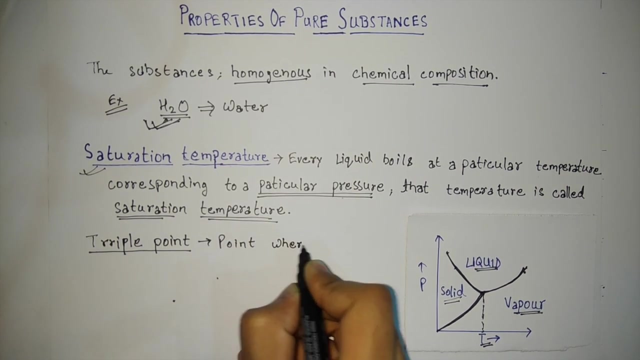 Now in this graph you can see there is an intersection of three lines coming at one point. This intersection point has a temperature. this is known as critical temperature and this point is known as the triple point. Hence, the triple point is defined as the point where all the three phases of water 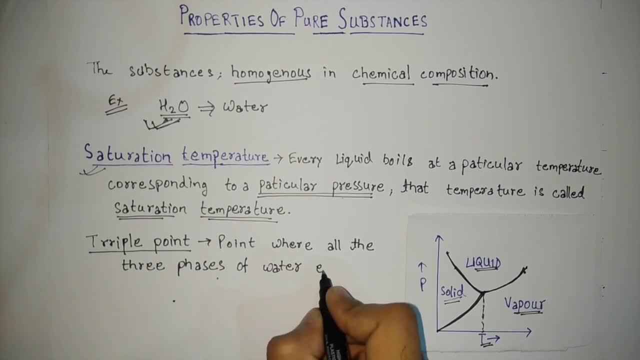 or pure substance exist. Now in this graph you can see there is an intersection of three lines coming at one point Here you can see at this point liquid phase also exist, vapor phase also exist, as well as the solid phase. That is why it is known as the triple point and the temperature corresponding to triple. 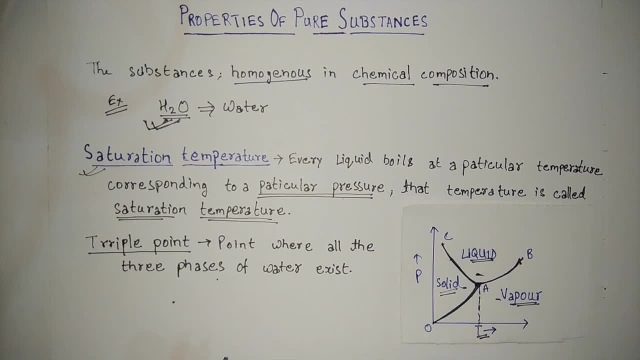 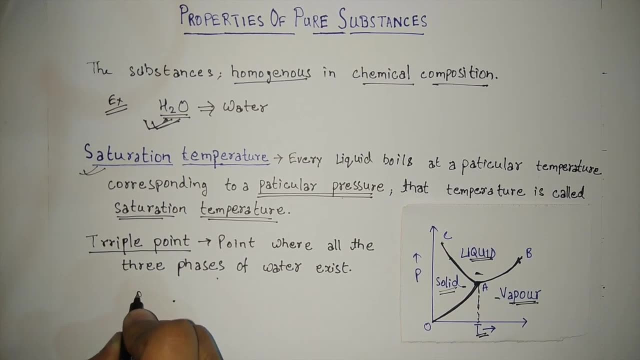 point is known as critical temperature. If we name the line as O, A, B and C, The line OA represents sublimation line, sublimation line. The line AB represents vaporization line, While the line AC represents fusion line. 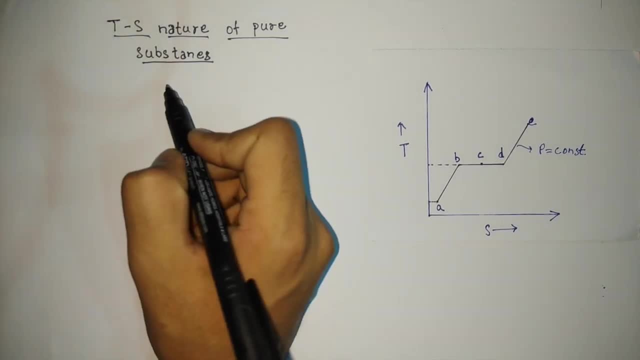 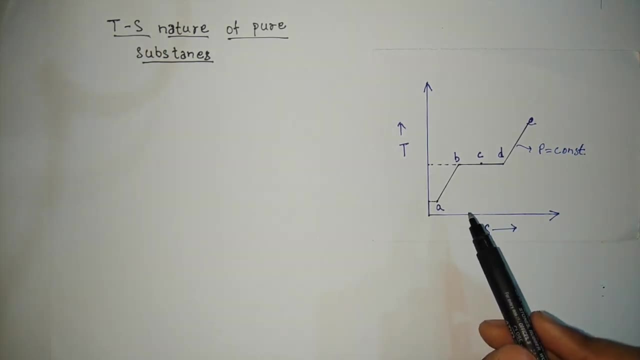 The next is TS- nature of the pure substance, Where T is temperature and S is entropy. Here is a graph that shows the nature or the variation of pure substance between temperature and entropy, plotted at constant pressure. As the temperature increases, the entropy will increase, but after a certain point the temperature remains constant, while the entropy increases and the temperature increases. 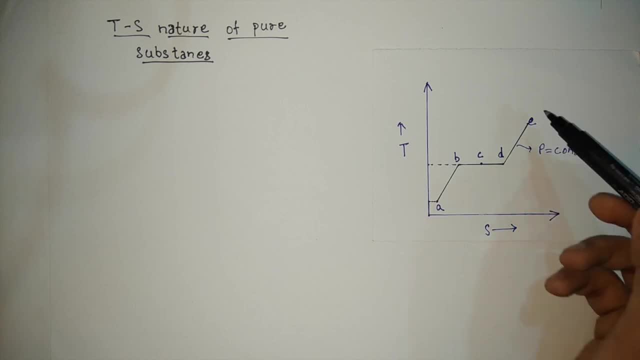 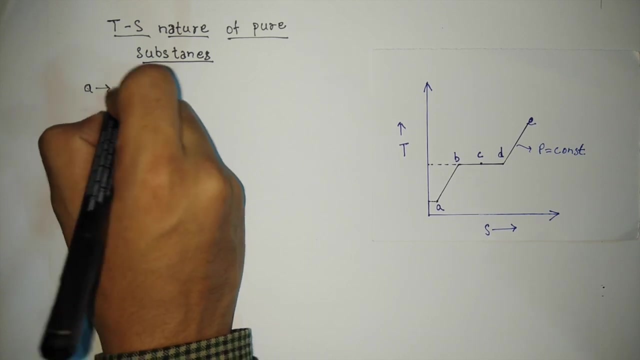 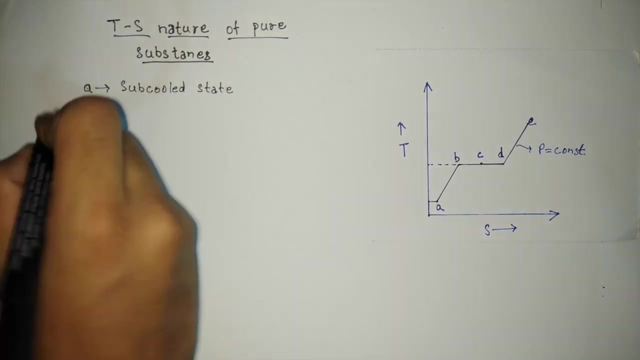 And then after that, when entropy increases, temperature also increases. So we get points A, B, C, D and E. There are several points on this graph and these points are defined as. Point A is defined as subcooled state. That means the initial point, Point B, is defined as saturated liquid state. 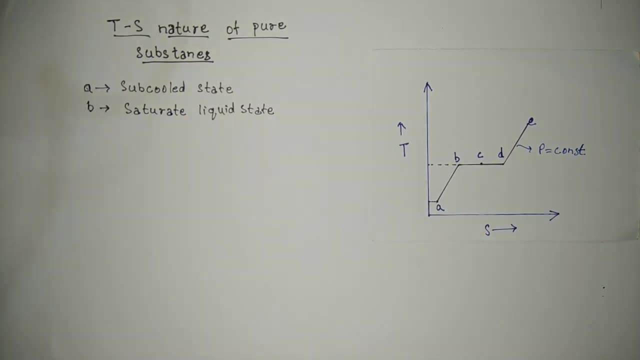 That is the point from which the liquid will start changing into vapor. Up to this phase The substance, The substance, is in liquid state. Between B to D it is liquid plus vapor, and after point D it is totally vapor. So point C is defined as liquid plus vapor state. 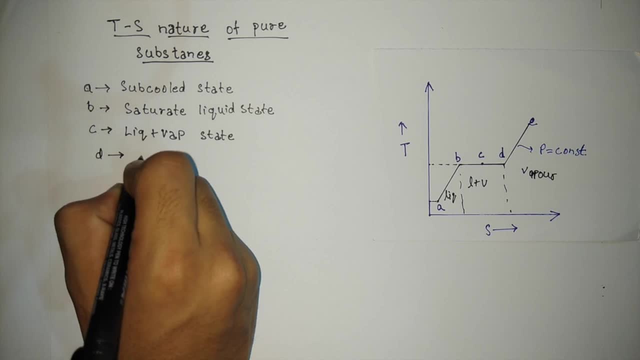 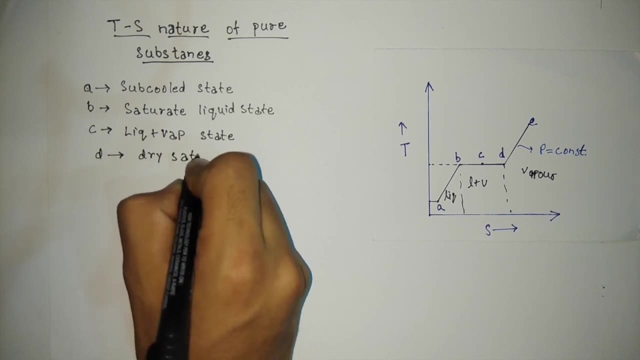 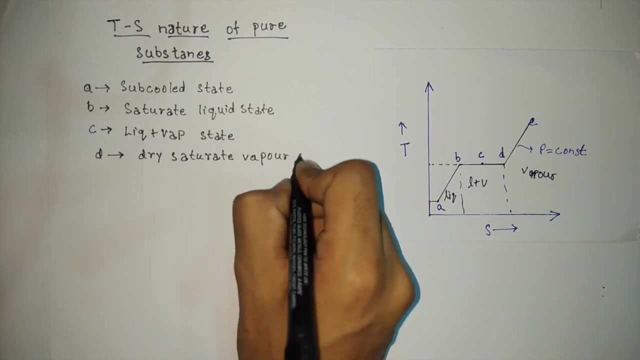 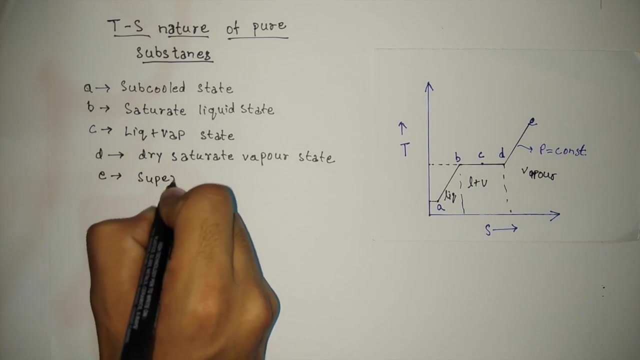 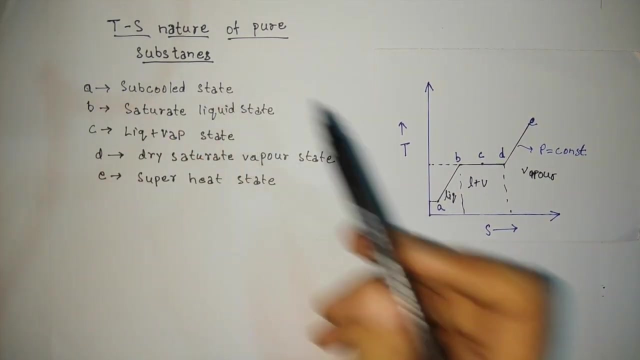 Point D is defined as Point C is defined as liquid plus vapor state. Point D is defined as liquid plus vapor state- Dry saturated state, While point E is defined as super heat state. point a is sub cool state, that is, the initial state of the liquid changing to vapor. point b: 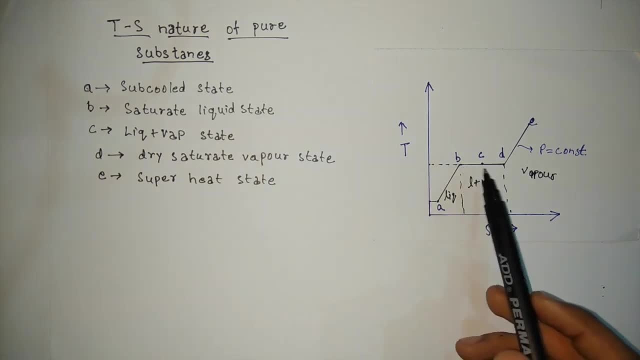 is the saturated liquid state. that is the point from where the liquid will start changing into vapor. point c is liquid plus vapor state, that is, at this phase the liquid and vapor coexist. point d is dry saturated vapor state. that means the point from which the liquid completely. 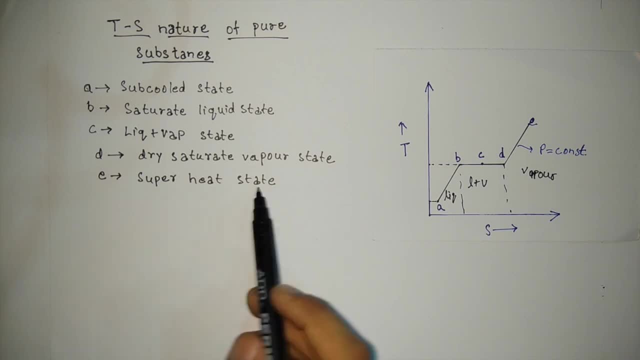 transforms into vapor and point e is the superheat state, that is, the final state of the vapor. the temperature at b is equals to temperature at c is equals to temperature at d, is known as the saturation temperature. the heat between b to d is known as latent heat. 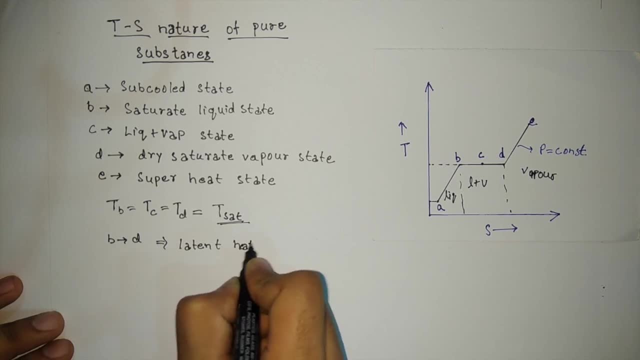 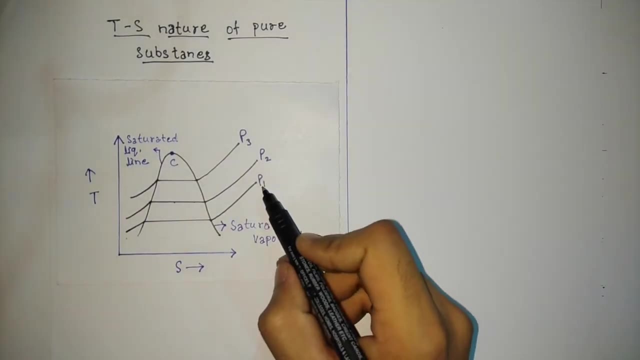 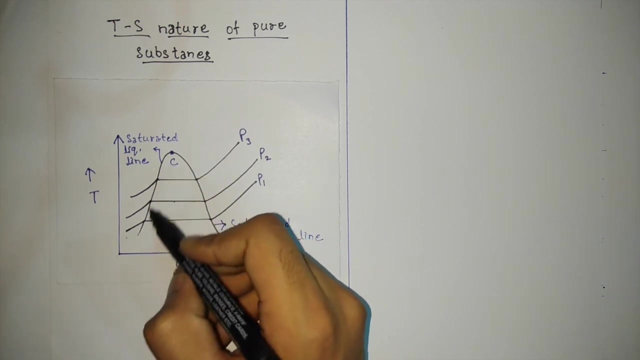 if you draw the ts curve for several pressures- that means p1, p2 and p3- we will get the graph like this: at p1 it will be like this, at p2 like this and p3 like this: joining all these points we will get a dome like shape. 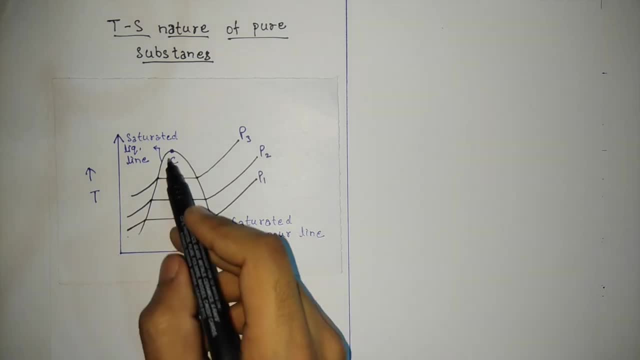 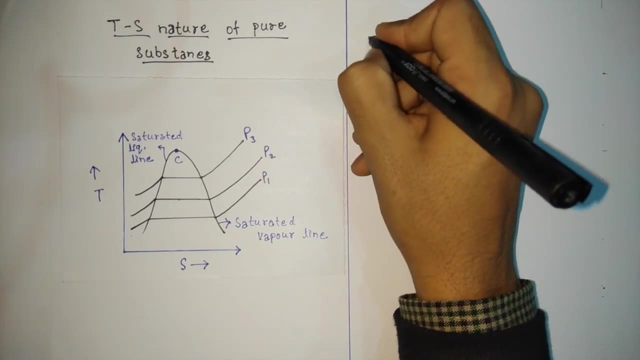 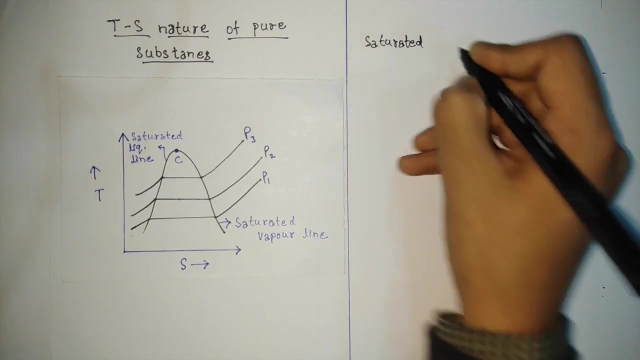 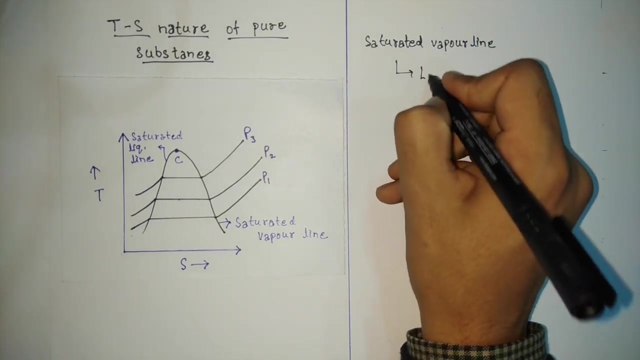 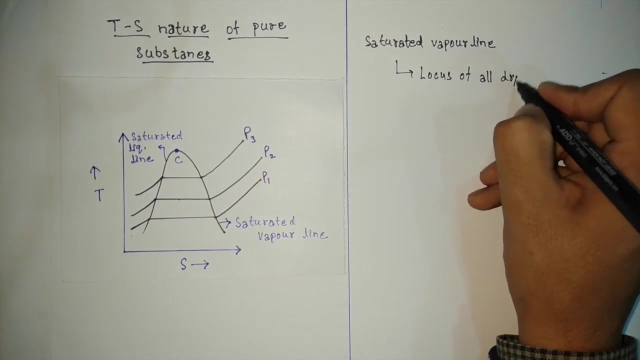 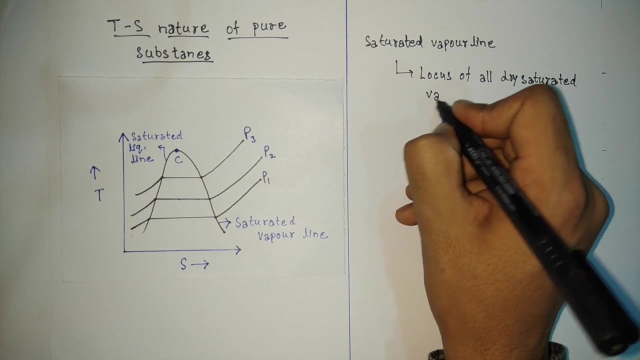 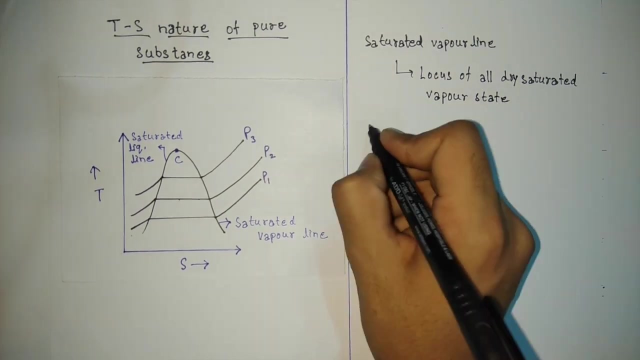 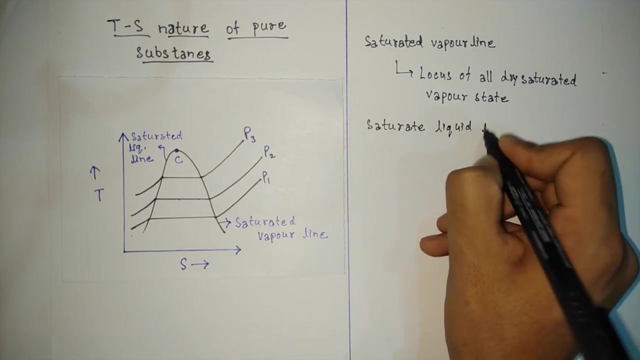 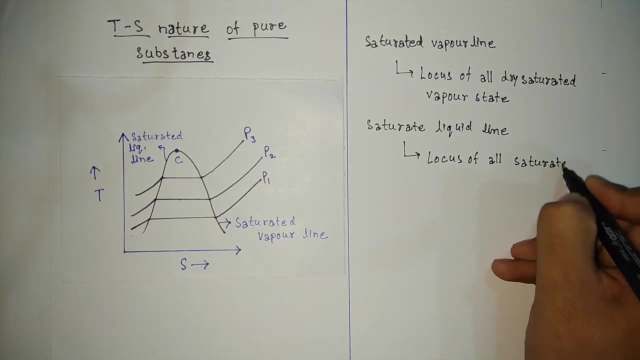 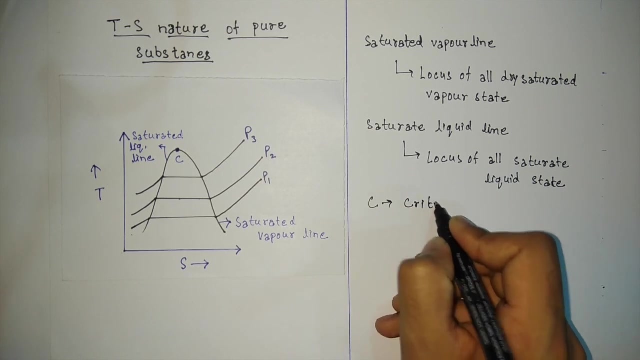 this part is known as saturated vapor line, while this part is known as saturated liquid line. so saturated vapor line is the locus of all dry saturated vapor state, while saturated liquid line is the locus of all saturated liquid state. The point C, that is, the peak point of the dome, is known as critical point, that is, beyond. 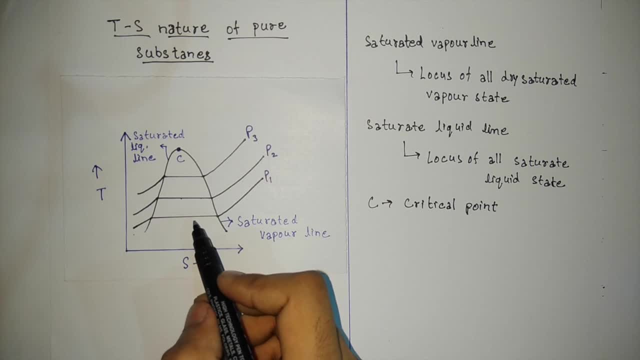 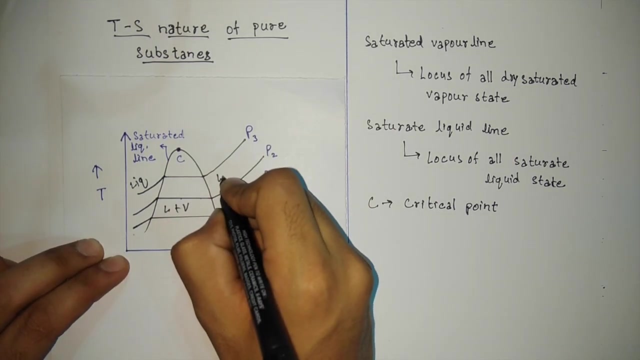 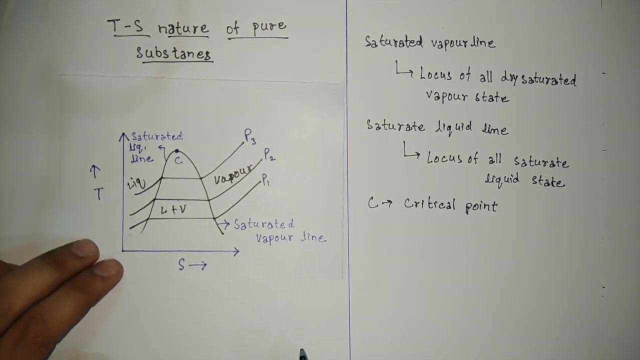 this point the latent heat will be zero. that means the liquid will directly change into vapor without going into liquid plus vapor state. This phase is the liquid phase. This phase is liquid plus vapor phase, While this phase is fully vapor phase. So, beyond critical point, the liquid directly changes to vapor without going to liquid plus. 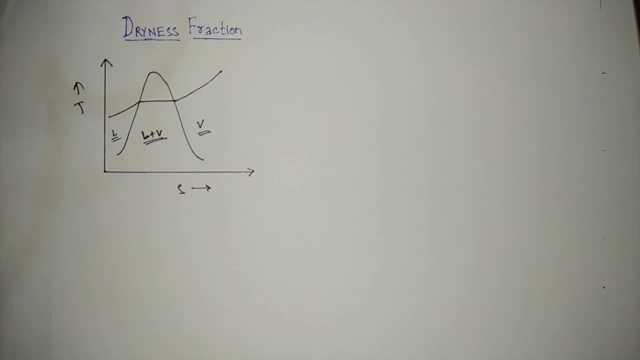 vapor phase. The next topic is dryness fraction. It is denoted by small x, The amount of dry steam present in total amount of wet steam. That is, x is equal to 0.. x is equal to m v by m l plus m v. 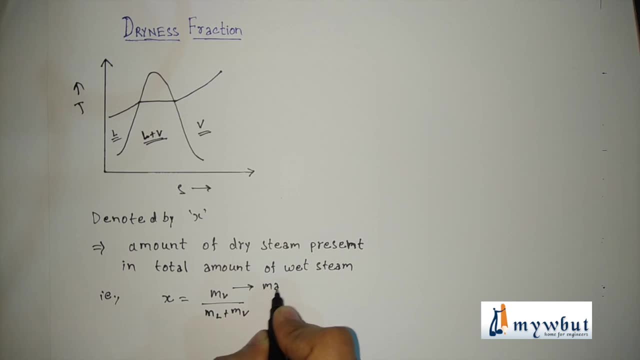 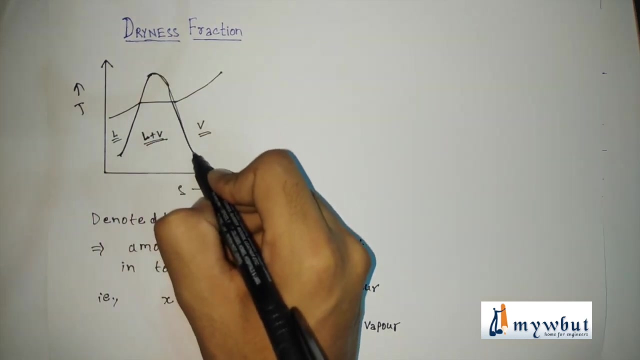 Where m is the mass of dry vapor, m l is the mass of liquid Or wet vapor. Clearly, with the definition you may have understood that X or dryness fraction can only be defined between these zone, that is, inside this dome. This dome is known as vapor dome because inside this dome only the liquid as well as the vapor. 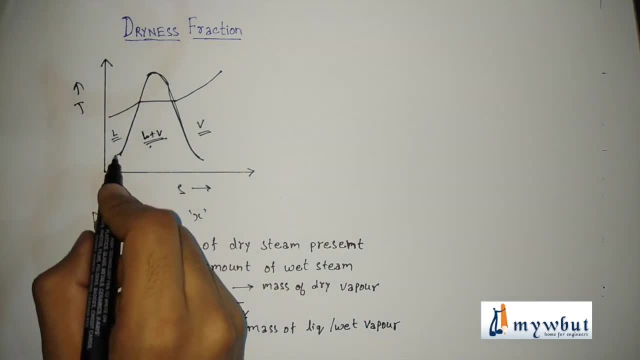 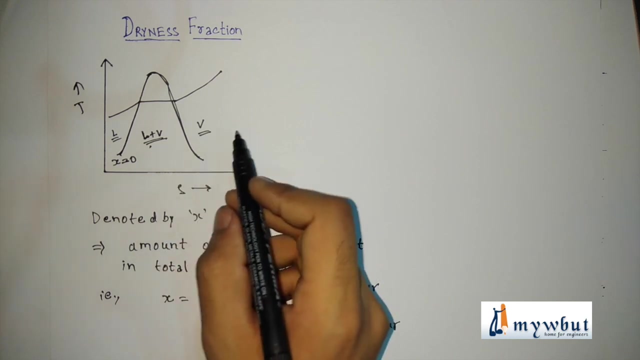 phase exist. So at the starting point it is all liquid. that means the X value is zero because there is no dry vapor is present. the mass of the vapor is zero and at the right side the all substance is converted into vapor. that means the X is equal to one. that means the vapor. 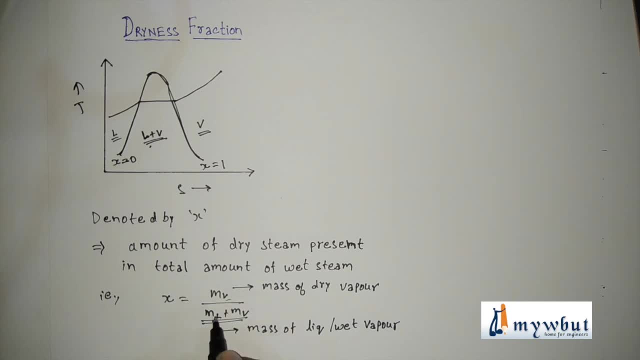 mass is totally equal to the liquid, the liquid mass will be zero. so the vapor mass is the total mass of the steam. So the X is equal to one. between these, X is equal to zero and X is equal to one. the dryness fraction varies in inside this dome. 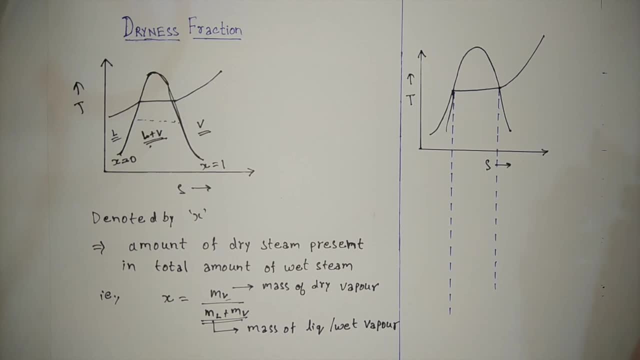 Now consider the TS diagram once again. here we will know some important relation. while calculating the dryness fraction, The end point of the right hand side of the dome is represented by X If, while the left hand side is represented by G. so between these two entropy is represented. 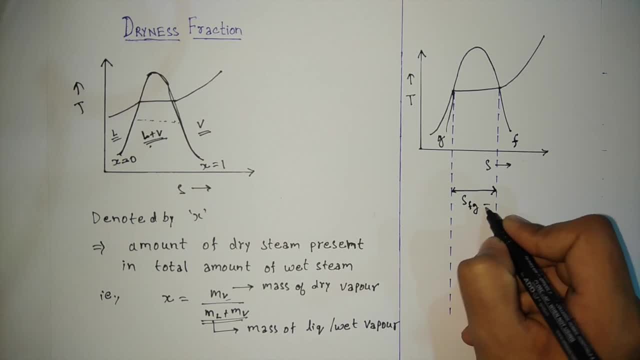 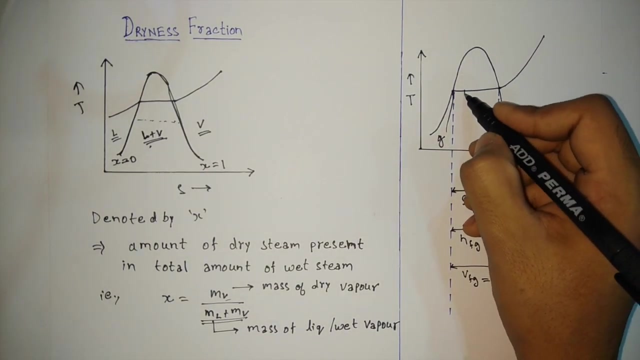 by SFG, which is equals to SF minus SG. similarly, if on the X axis we have enthalpy, then HFG that will be equal to HF. Similarly, for volume, VFG will be equal to VF minus VG. If we need to find out the value of Entropy or enthalpy between or inside this tone, we 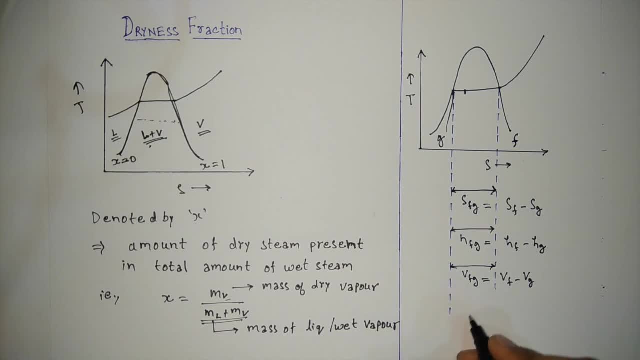 use the relation Suppose writing. for entropy, It will be: a. sex is equal to SG plus X SFG. for enthalpy, it will be: HX is equals to HG plus X- HFG. the values of SFG, HFG will be calculated through the steam table. 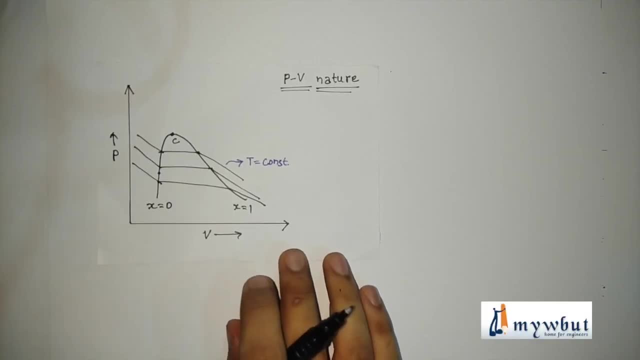 the next is PV nature of the pure substance, that is, pressure volume nature. so far we learned PT and the TS nature of the pure substance. now the PV nature of the pure substance. here the dome is shifting more towards the right side and it is drawn at the constant temperature. and notice the difference that the 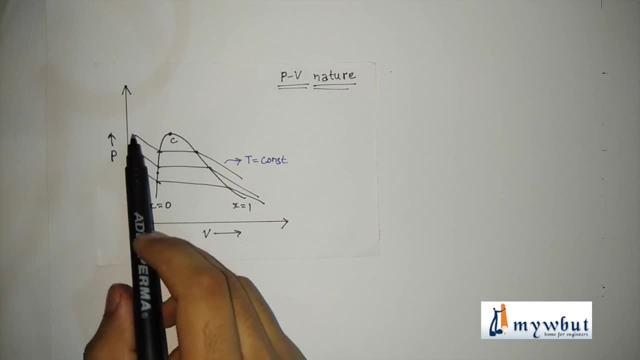 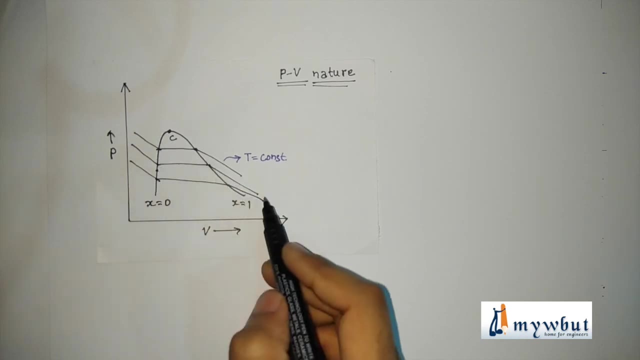 temperature pressure is decreasing in nature. that means it is coming from up to down and the shape of the dome is slightly changed. on the right hand side, left hand side is quite similar, while on the right hand side it is more shifting towards the right side more so. this is the nature of the pressure volume curve of the pure 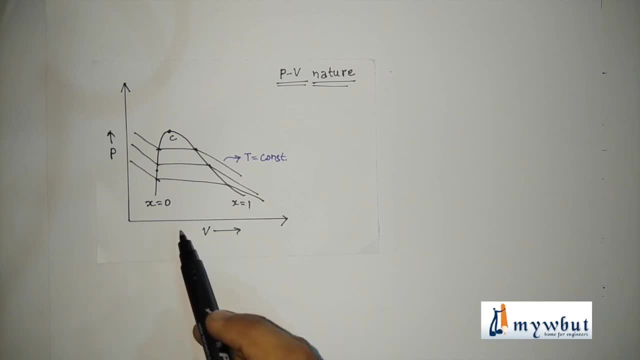 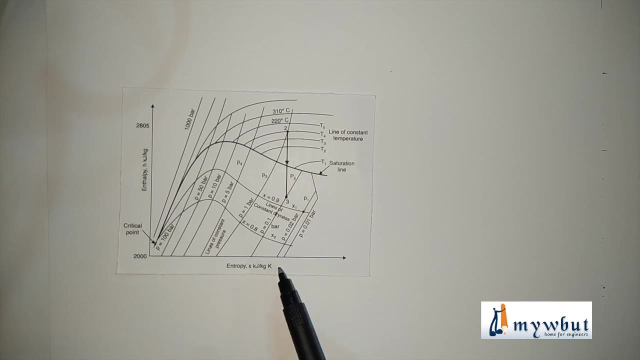 substance. the next is HS curve. that means enthalpy versus entropy curve. this is also known as Mollier's chart. the dome here is having shape like this: it is drawn at the constant temperature line, which is shown here, and the constant pressure line, which is shown here. now the dryness. 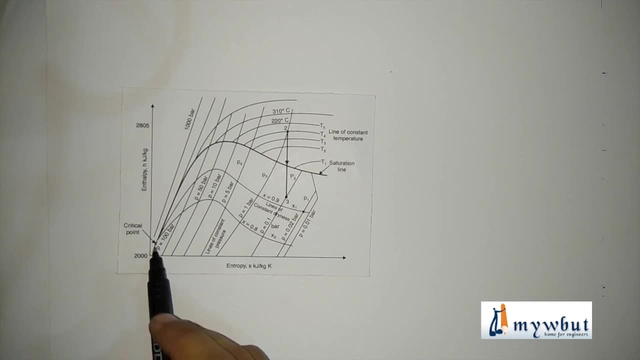 fraction changes from here X equal to 0 to X equal to 1. for example, in this diagram it has shown the dryness fraction line is changing from here in the mask O さn line of x equal to 0.8. here it is shown x equal to 0.9. now this diagram is very important to find. 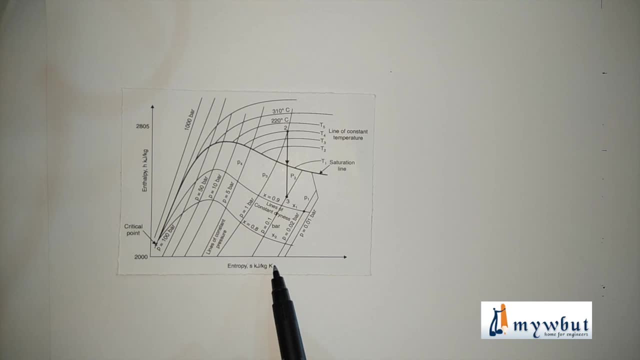 out the value of enthalpy or the entropy for a specific given temperature and pressure. suppose the temperature is given, consider 220 degree celsius- and the pressure is given as 5 bar. so considering the 5 bar line and 220 degree celsius line.